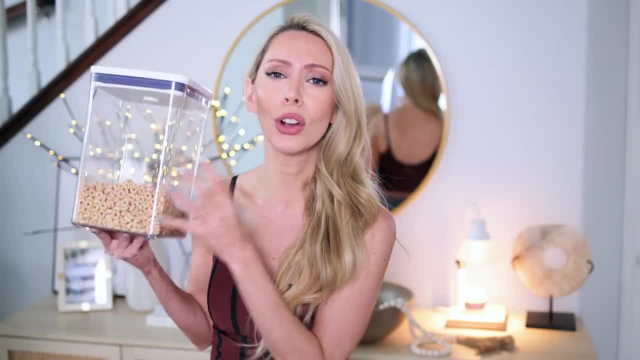 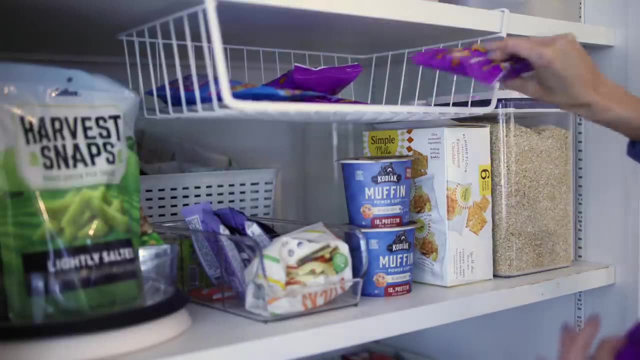 go of my fantasy self, who had a perfectly gorgeously organized pantry in these pretty containers, And instead face reality and have a system that actually works. So go around and test this out around your house. Are your organization systems so seamless, so simple that you can just toss? 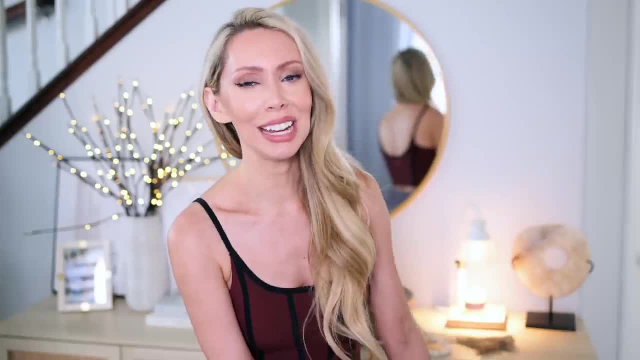 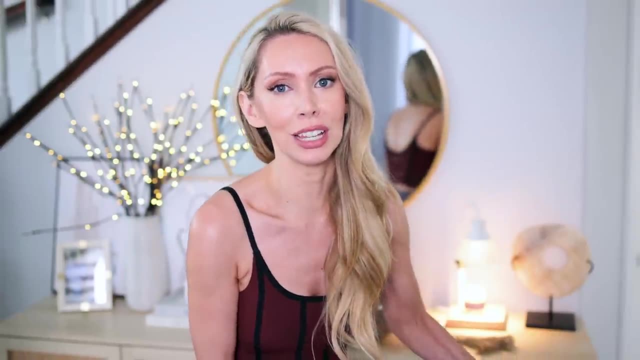 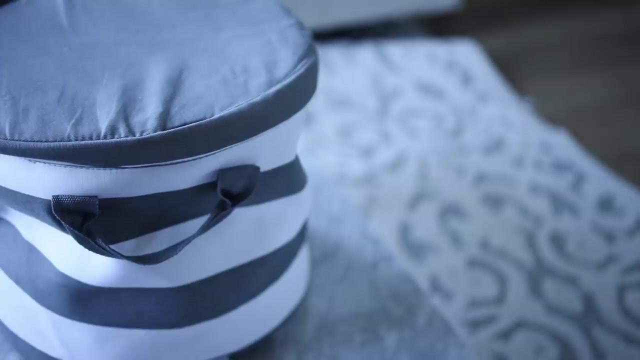 and go. If so, it passes the test. The next tip to maintaining an organized home is to make things easier for yourself and your family members to keep things clean. So, for example, with my kids, my son in particular. he loves playing with Legos, So I got him this smart toy bin. So this makes it. 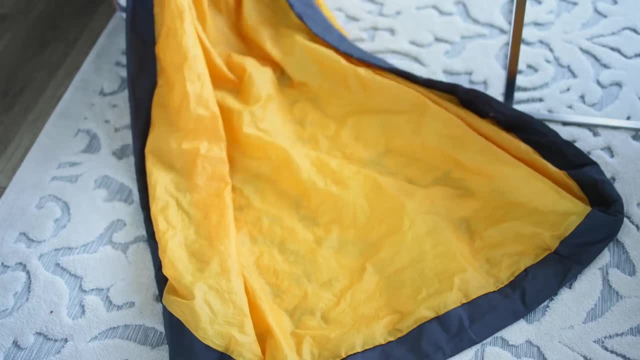 easier, faster and more efficient. So I'm going to show you how to make it easier for yourself and your family members to keep things clean, faster and more efficient for him to clean up after himself. This bin: you can pour them out, and it has a mat, So he plays with the Legos on the mat. 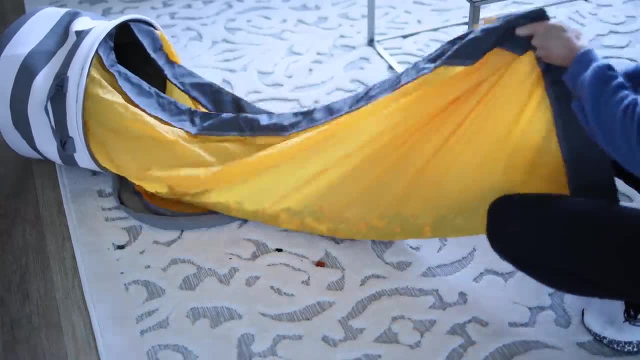 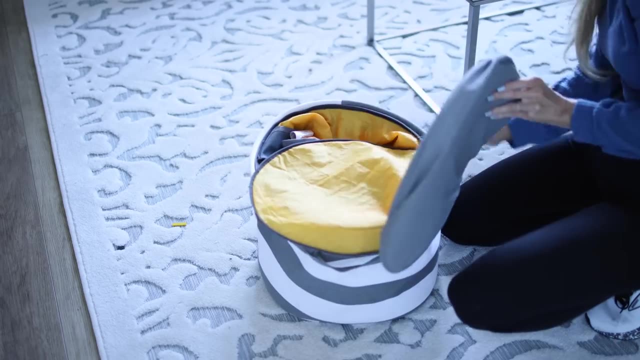 And when it's time to pick them up, all he has to do is pick up the mat and you're good to go. And this is not just for use with Legos. If your kids have any small toys where pieces are getting everywhere, they're getting lost. It takes forever to clean up. Work smarter, not harder. A professional. 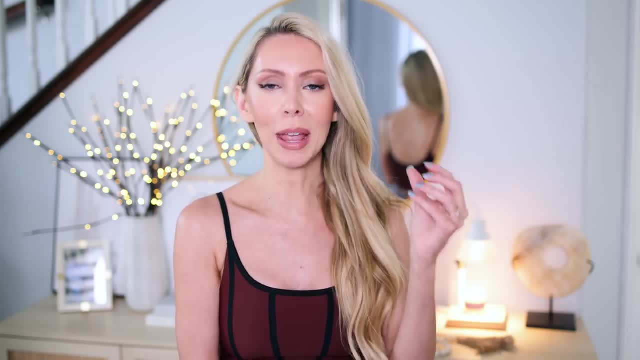 organizer named Karen Ford has a whole course on managing your cords. She's like: if there's one thing that you need to do to clean up, it's the legos. So she's like, if there's one thing that you need to do to clean up, it's the legos. So she's like, if there's one thing that you need to do to. 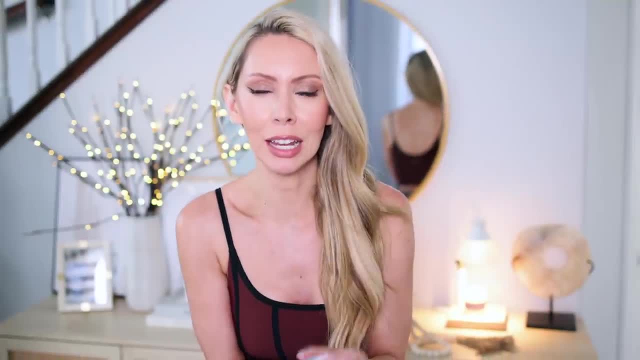 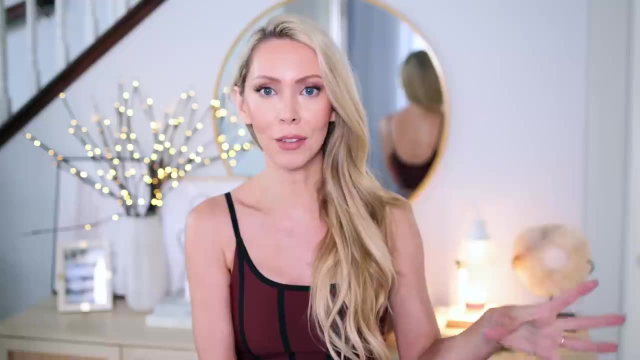 clean up. it's the legos. So she's like if there's one thing that you need to do to clean up, it's your cords, Because they are such visual clutter. And she has two items that she recommends. First one I already have. It's called the wall buddy. So instead of having your cords plugs all, 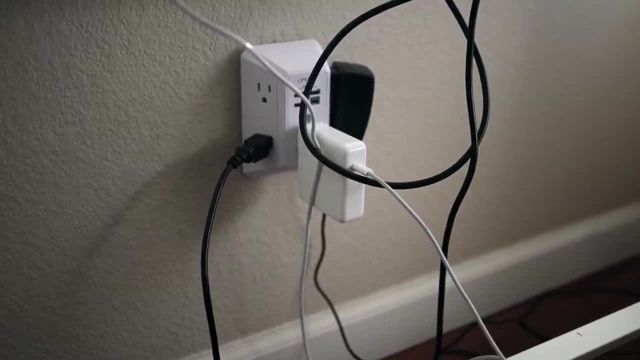 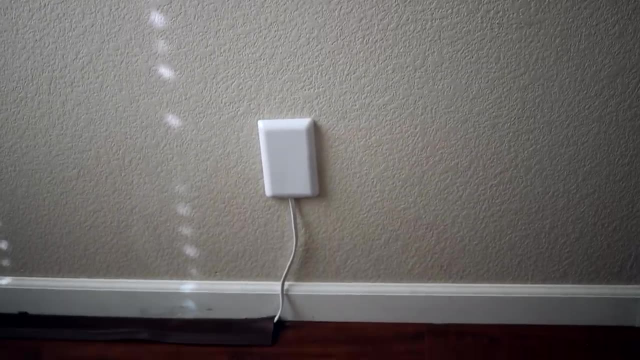 centralized on the outlet of your wall in a visible location. it just looks messy, cluttered. This is called the wall buddy. So you plug this into the wall and it has an extension cord built in. You put that behind a furniture item and then plug things in there. 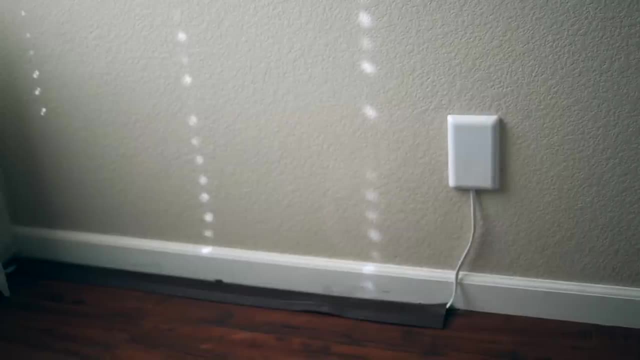 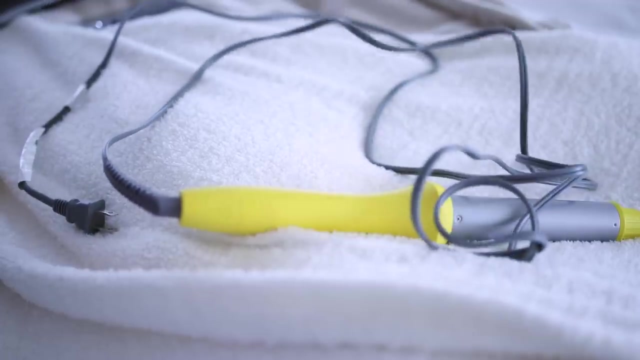 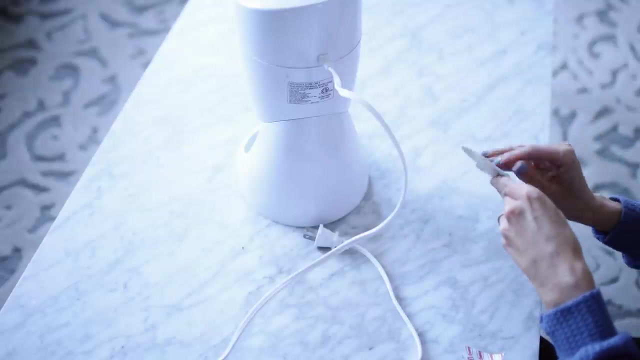 So you can't see the cords. It takes it from looking cluttered to clear. Another household cord nightmare that could be very easily solved are appliance cords. So now they make these command cord containers. They're specifically designed to stick onto multiple surfaces- any type of appliance or device you have, and contain the cord right. 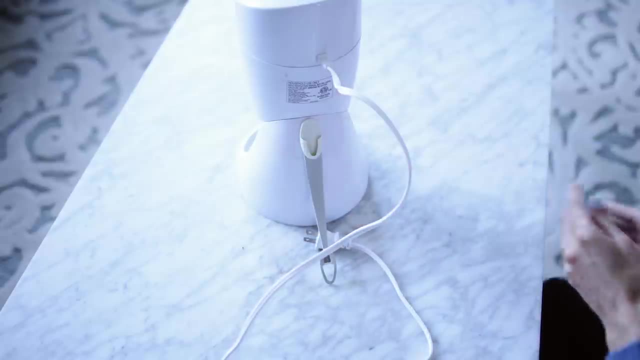 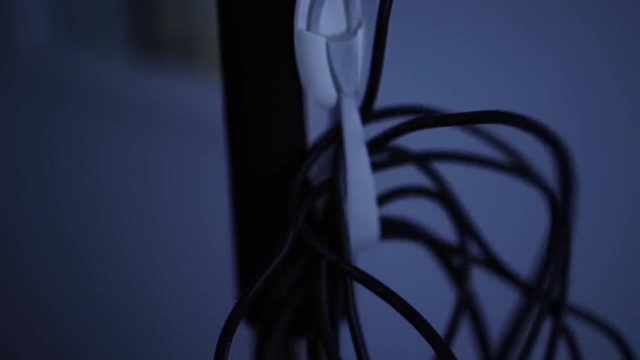 into it. You can also use these to hang like wreaths or garlands. I used to just use regular command hooks, but it wouldn't stay in place. The cord would fall off. This has the loop that you just secure in place, So the cord isn't going to go anywhere, And all of your 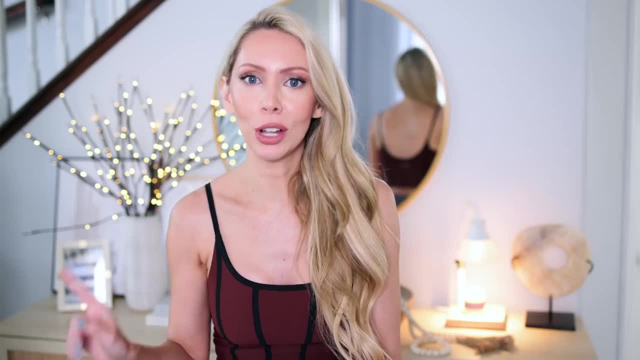 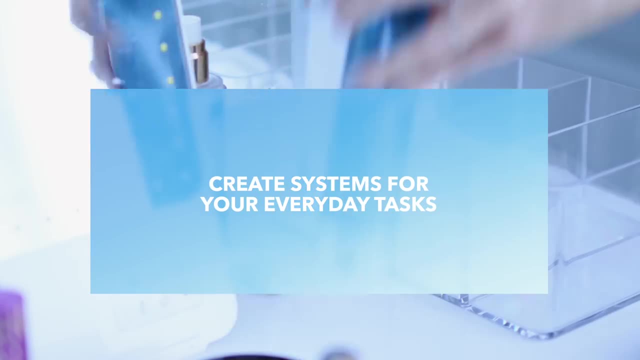 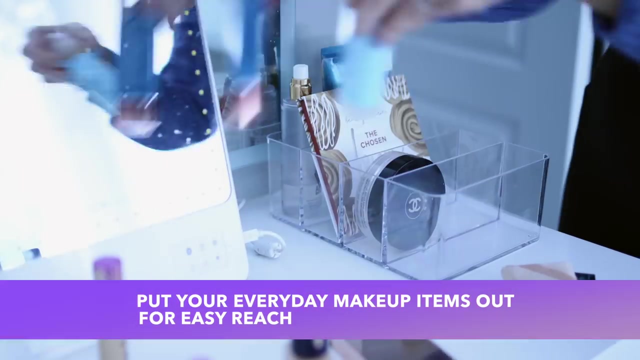 items cords are contained. An organizer named Scott Woods from Atlanta said that his biggest organization secret is to have systems for your everyday tasks. He recommends having one small organizing bin for all of your everyday makeup. He calls it your top shelf items that you grab. 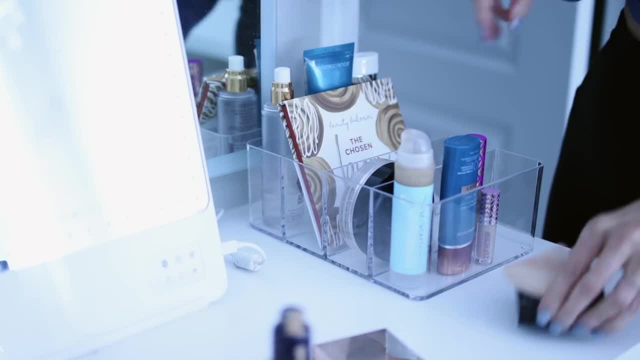 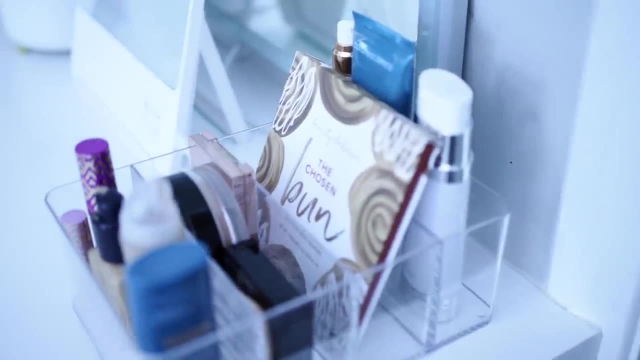 the most. put them all in here, keep it on your countertop, So not only is it making it faster for you to get ready, but easier for you to keep Everything clean and contained and organized, because it just comes out, use it, put it right back and it's right there within easy reach. Also, I got this new makeup. 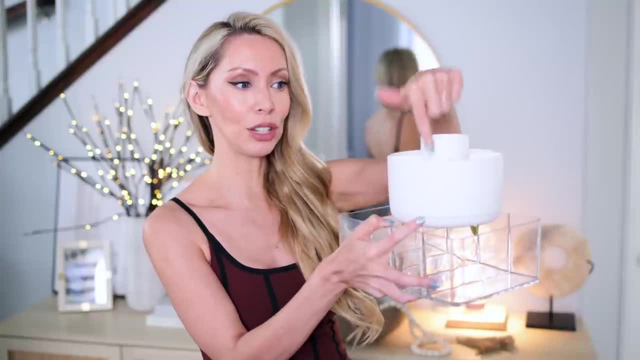 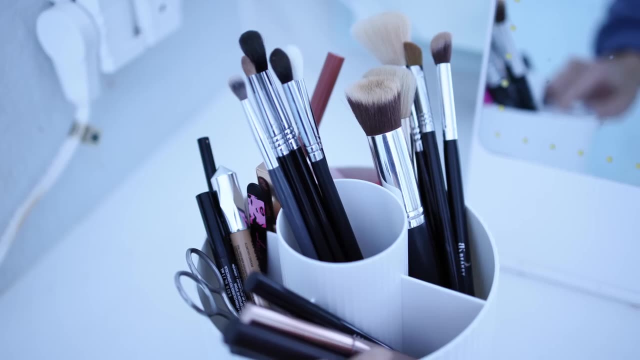 brush holder that I really like the design of this because you can sort your brushes. So I have face brushes, eye brushes. it twists so I can grab what I need, put it back easily. So these two right here have been game changers for my everyday. getting ready fast like 10 minute mommy makeup. 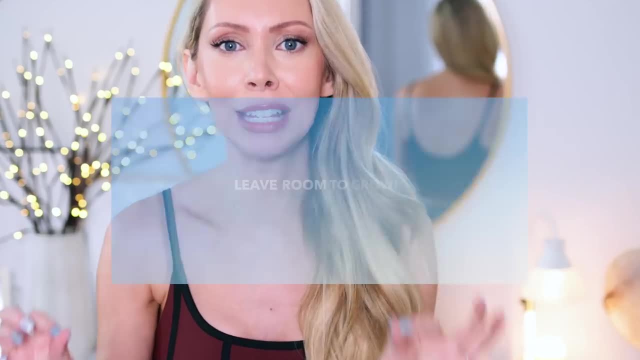 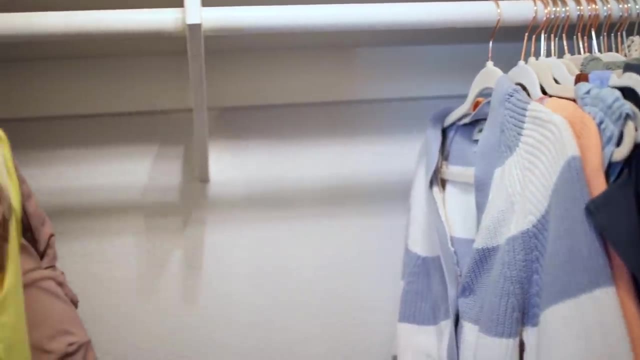 routine. Next organization secret is: you must leave room to grow. Any system you have in your house, there needs to be a lot of empty space. It is very tempting to fill up all your bins, get everything looking gorgeous and full and complete, But in doing that, 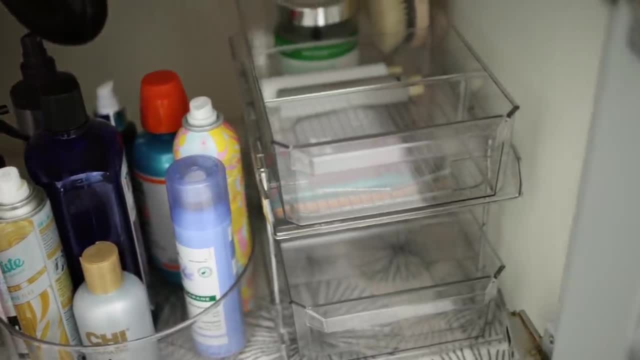 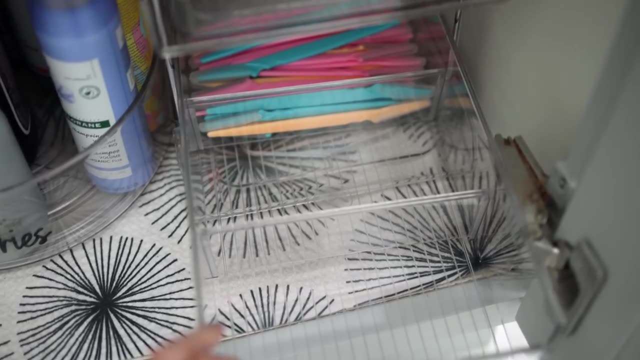 you again are setting yourself up to fail because life happens, You're accumulating more things. So if you don't have the extra space available, where are the items going to go? They're going to get shoved and crammed And before you know it, your system is going to completely fall apart. The next: 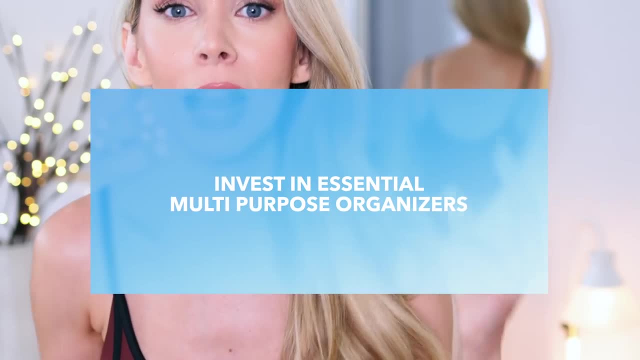 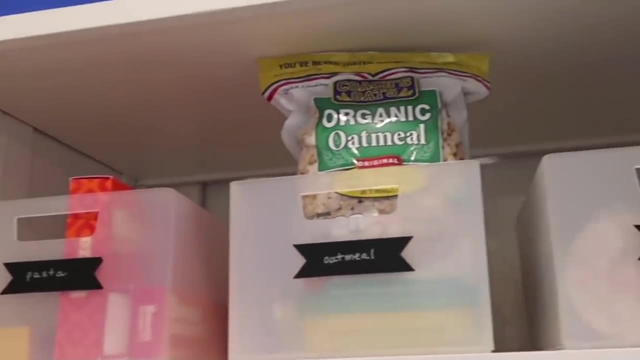 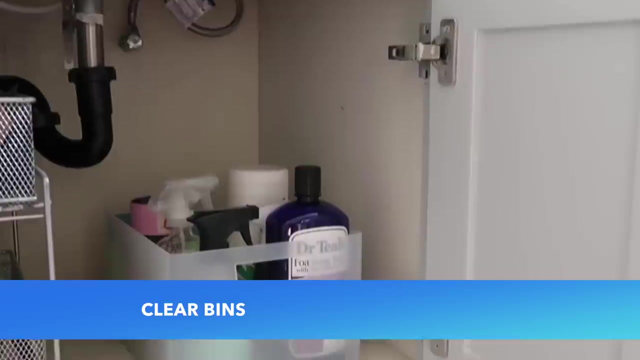 organization secret is to invest in multi functional, multi purpose organizers that you can use all around the home and get the most bang for your buck. And my little add on here is: have extras available so you can never go wrong with a clear bin. You can pretty much organize your whole house with just a clear bin. You can get a basic. 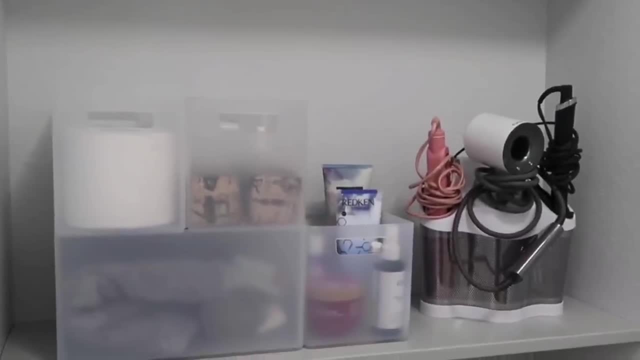 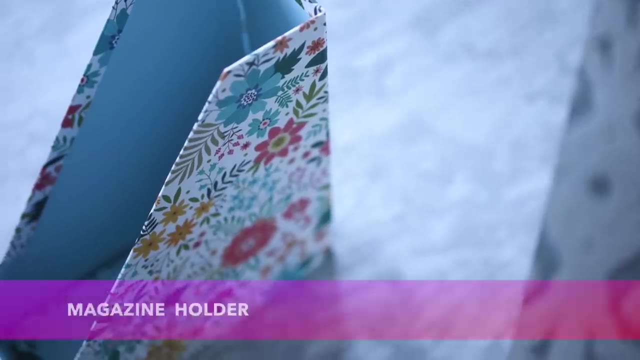 bin from the dollar store. These are my favorite because they're semi opaque. The next somewhat unexpected organizer that you can use all around your home in so many different ways is a good old fashioned magazine rack. Like I don't even use magazine racks for magazines, I just use them for 50 other things around the. 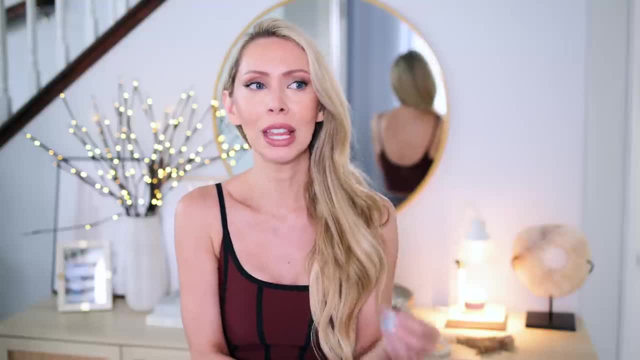 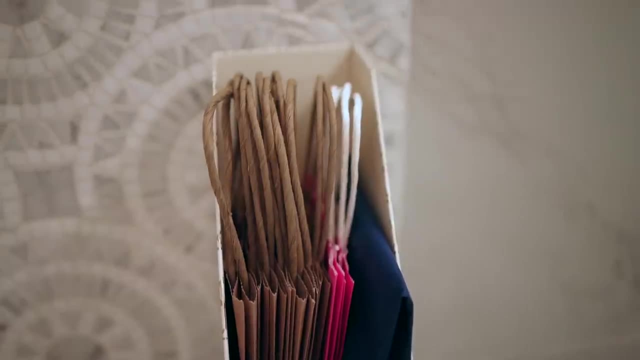 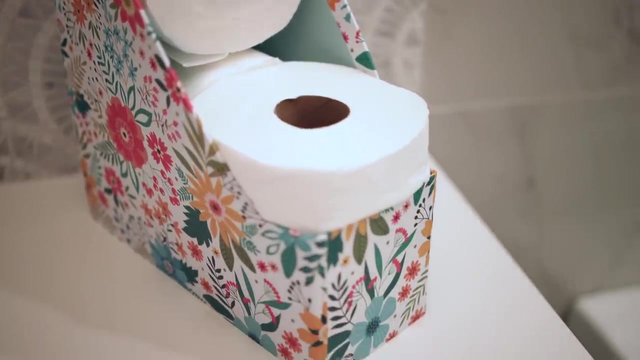 house. So I will show you a few of my favorite ways to use a magazine rack around your home. So for a gift wrap station, you put your gift bags, your tape bows, tissue paper in this toilet paper holder. we have the jumbo size toilet paper rolls, but regular ones will fit in here better. We have 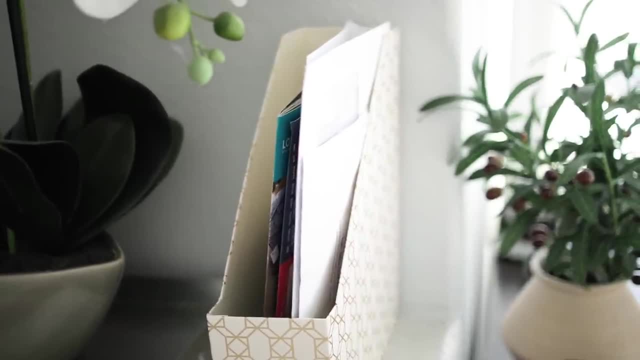 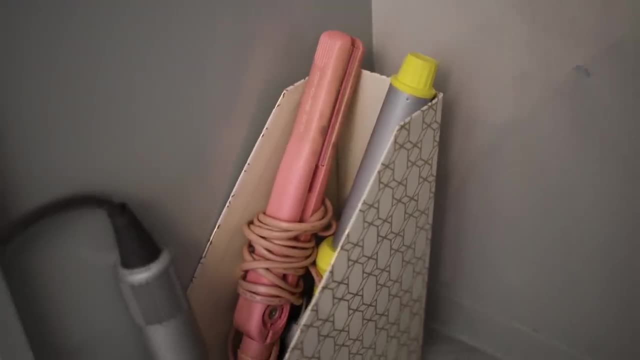 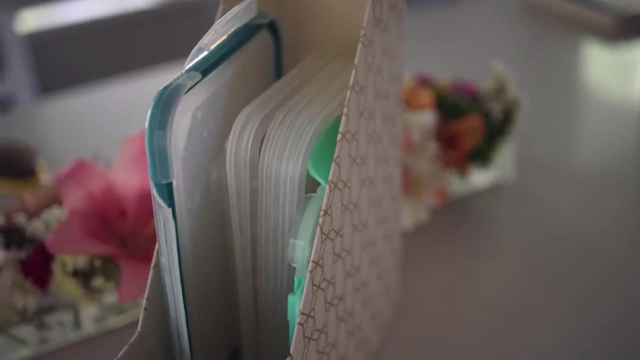 one as a little mail station by our front door, So important mail that we need to get to in the bathroom. I use this as my hot tools holder. So hairdryer, straightener, all of those things can just go right here under my vanity. you can use it to store your food container lids. they all stack up nicely. 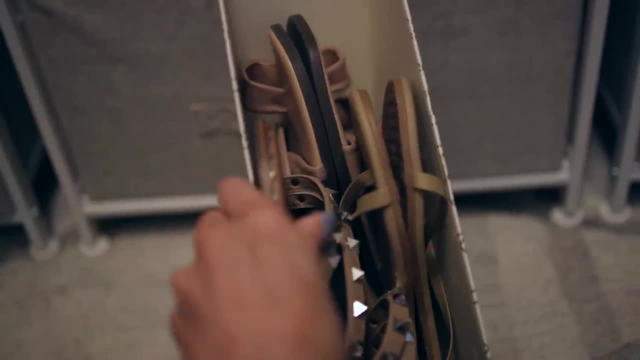 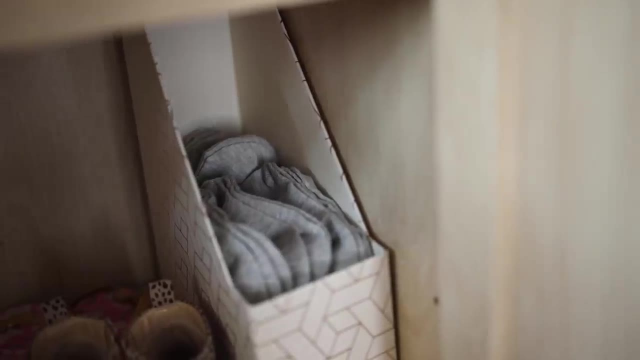 In your closet. you can use this for flip flops or your flat shoes. several pair will just fit in here and you can stock it in your closet. And probably my favorite way in the house: we use it to put our kids socks so it's easy for them to grab socks. They have these holders in a ton of. 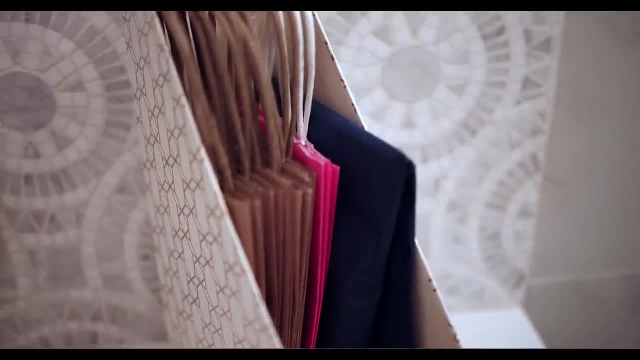 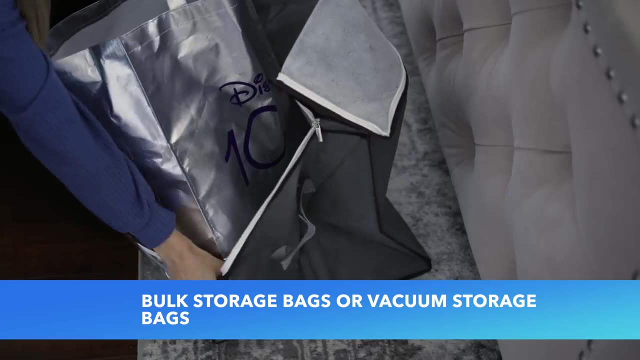 really pretty patterns. They're super affordable And, as you can see, very versatile. And then these are bulk organizer bags, good for storage. So anything that you are not currently using, that you don't need to take up valuable real estate in your home, put in these large storage bags. 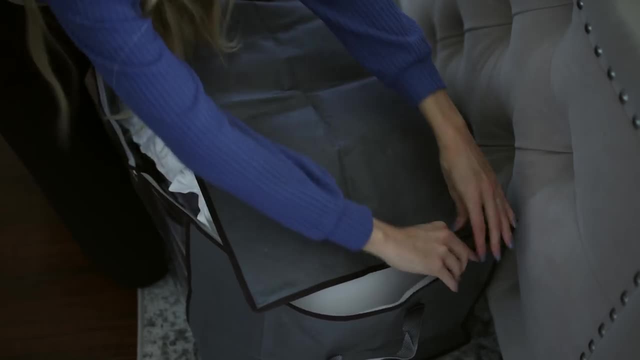 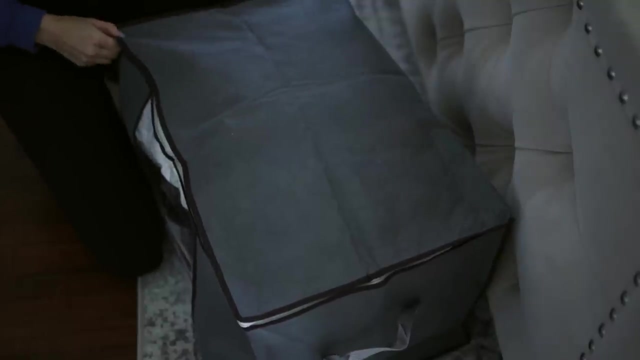 and put them in your garage or other storage space So they're not taking up space in your home. And what I like about these: they're big, they expand and they have the clear center So you can actually see what's inside. Next pro tip that's going to be your best friend are labels. 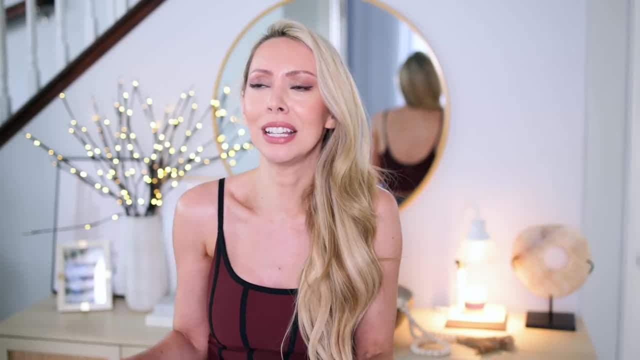 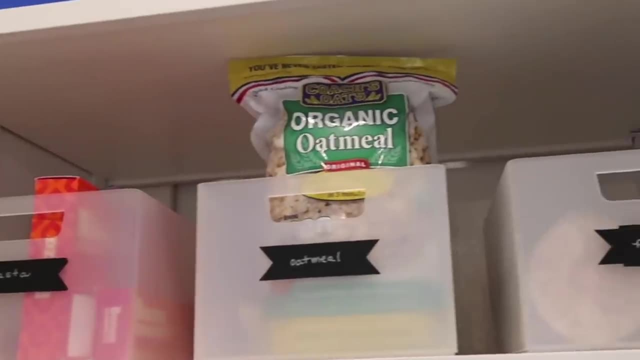 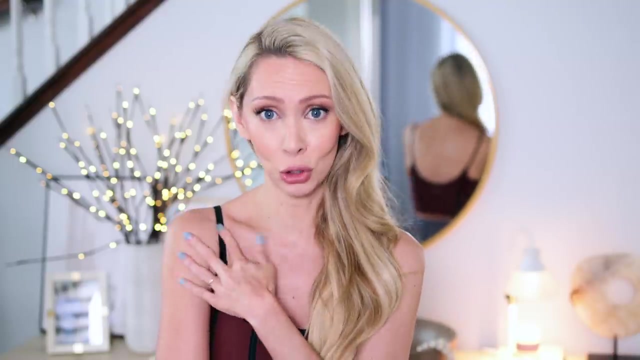 Any good professional organizer is going to tell you the importance of labeling. But what labels allow you to do is maintain the system and allow other people in your household to know where things go. Because, true story, Ryan, my husband asked me the other day where the scissors are. 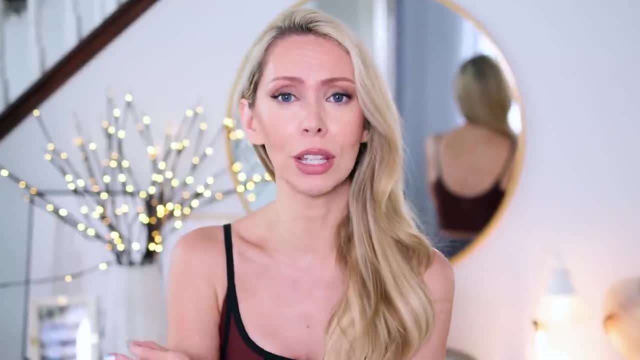 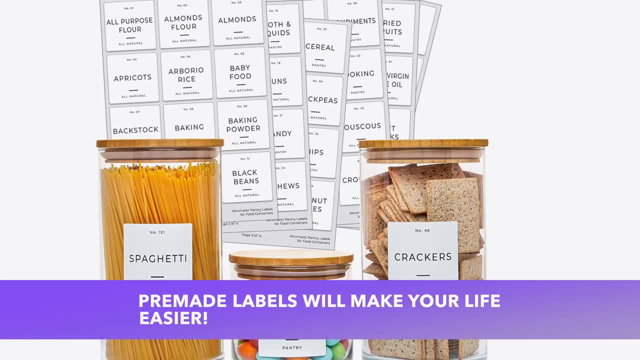 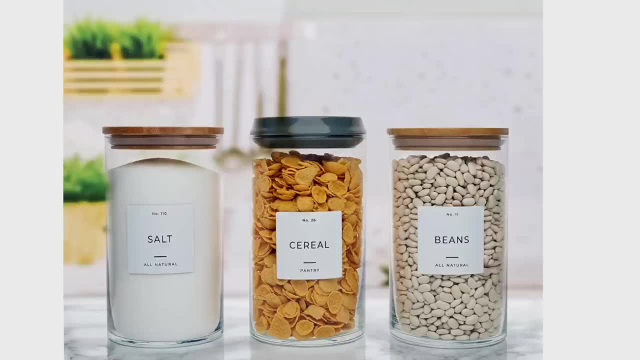 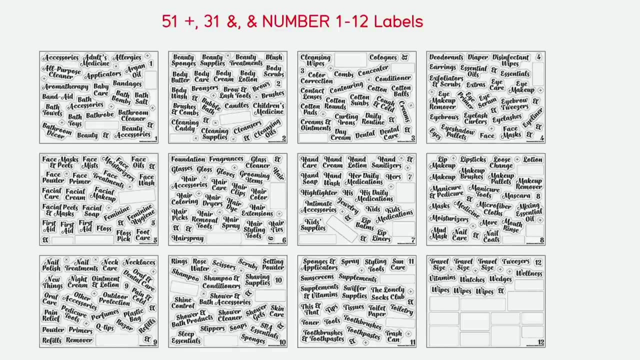 the trouble of getting a label maker and getting ink and the paper and it running out and printing them out yourself. It's so much easier just to get your labels and they have them in such pretty fonts, They look so professional and you just stick them on and you're organized. These are 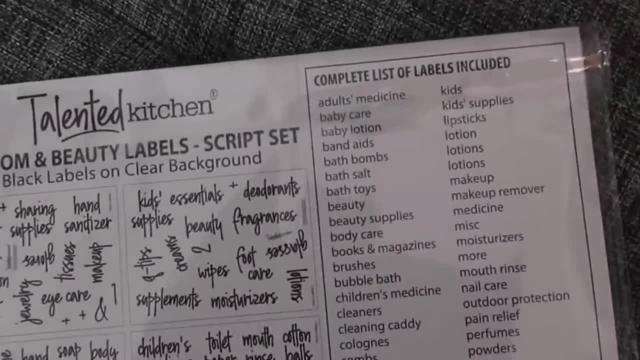 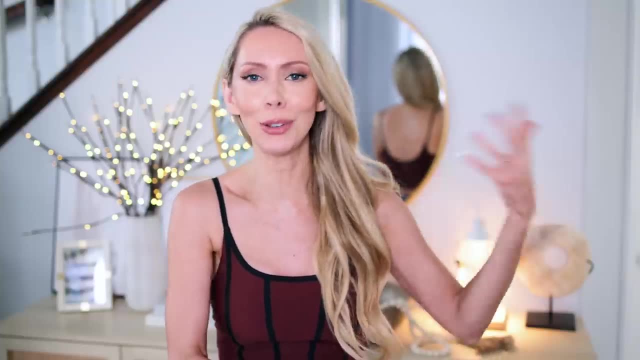 especially useful in the kitchen, the pantry and the bathroom room. I found just to maintain systems. Now, these last few tips all come from a professional organizer who is a YouTuber. Her channel is called Clutterbug. I will link her down below. 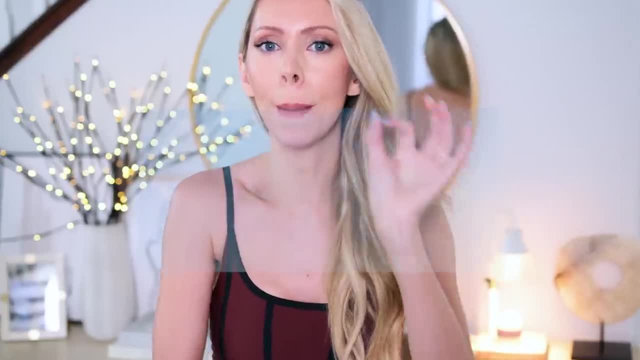 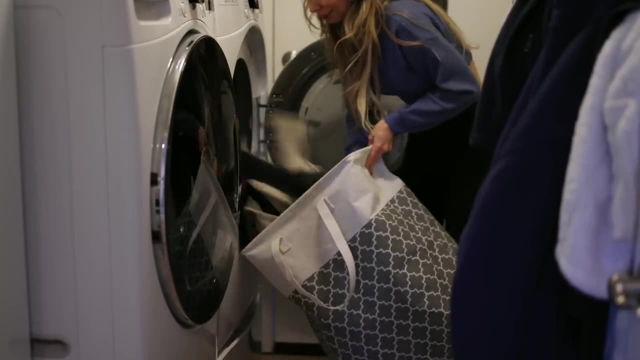 I love some of her tips, So one of them is called the one minute rule. She says that if anything is going to take you under one minute to either put back, organize, you do it and you commit to that- And I've heard this tip before as reference in like doing your work. So if it's going to take 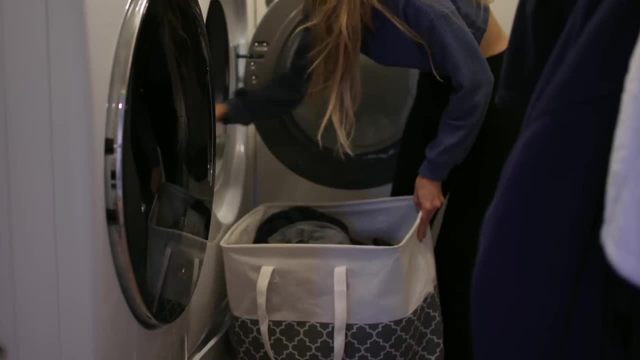 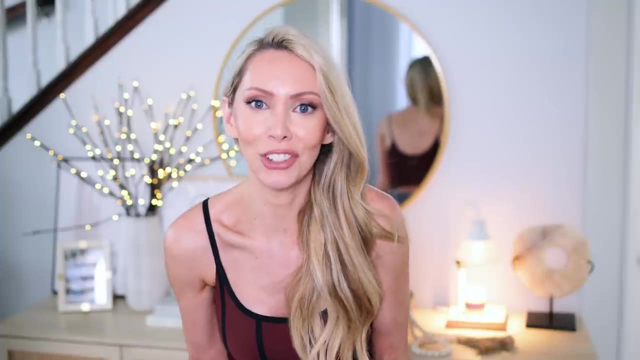 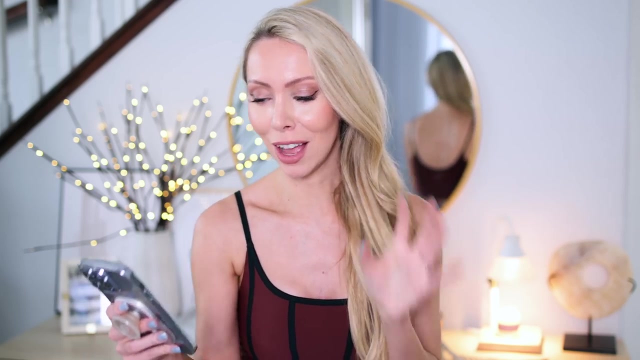 under a minute to reply to an email, do it right then, versus putting it off to doing later. So use that same approach to maintaining your home organization. If it's going to take under a minute, just bite the bullet. Just do it now and don't delay. And last tip from Clutterbug that I 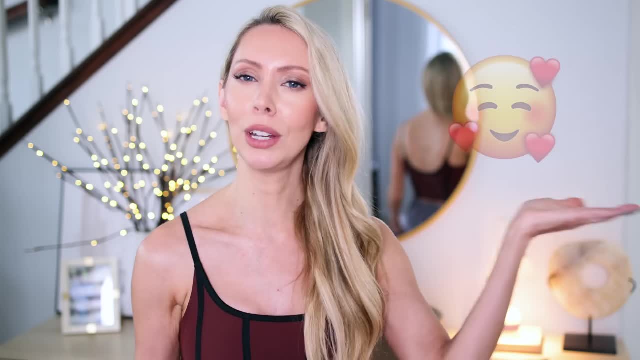 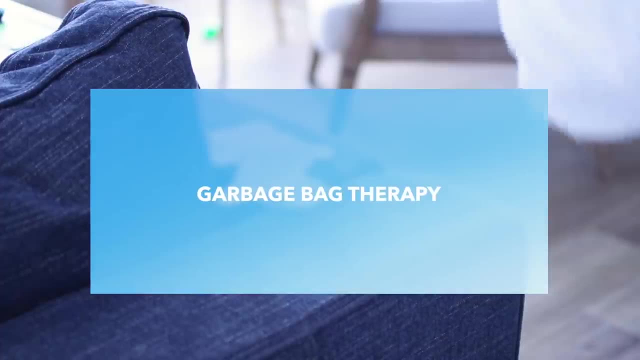 love, and I'm going to challenge every single one of you who's still watching. leave this emoji, so I know you're still watching. I'm going to challenge all of us, including myself, to do right now- And it is called garbage bag therapy- Get one garbage bag right now, right after this video, Get a. 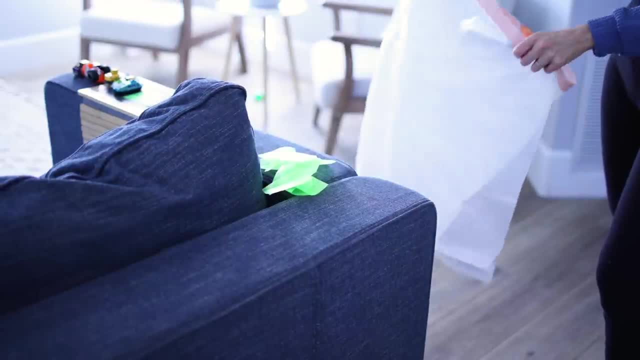 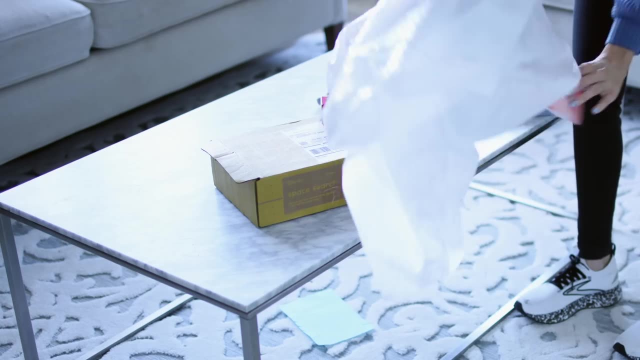 garbage bag. go around your house and try to fill that entire bag. Go through your drawers, throw away things That are expired, trash you're not using. You want bonus points. get two garbage bags- one of trash and one to donate- And just by committing to doing this right now, right after this video, you will 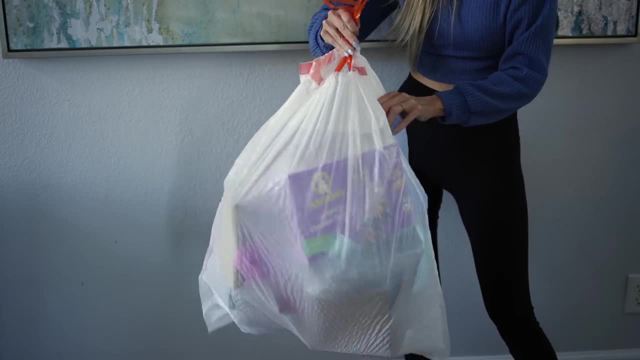 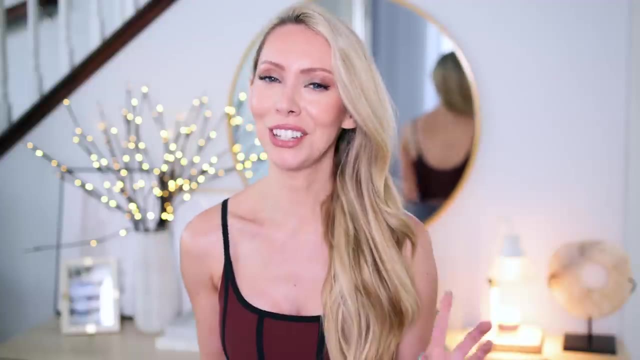 have accomplished something and you are well on your way to having a clean and organized home, So I hope you liked these tips that I've collected from some professional organizers. I will have everyone linked. If you did enjoy this video, make sure you're subscribed to see future videos from 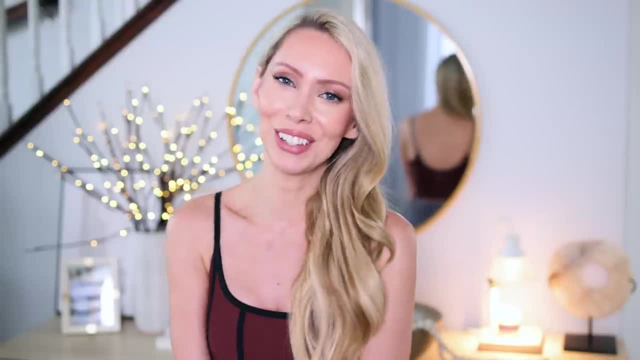 me And, with all that said, thank you, as always, for watching and I will see you soon with a new video. Bye.